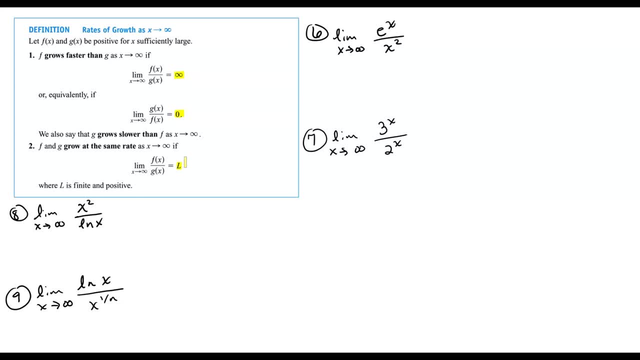 So let's go ahead and take a look here At number six, we're going to take the limit, as x approaches infinity, of e to the x over x squared. So you might look at this and say, well, how would I evaluate this limit? Well, I would tell you that the best approach for this is probably 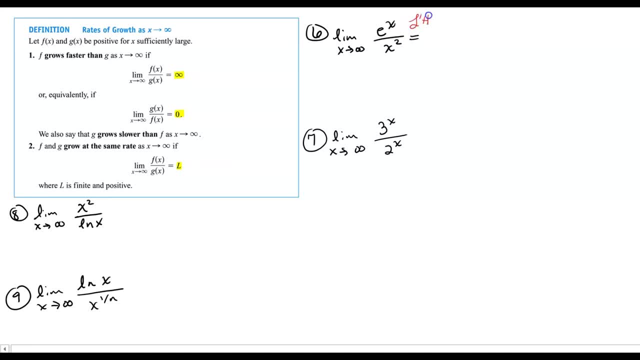 to apply L'Hopital's rule And, if you recall, L'Hopital's rule tells you that you take the derivative and you'll take it successively until you can evaluate it to see what exactly the limit may be. So let's take a look here at this limit. I'm going to take the derivative. Now, the derivative. 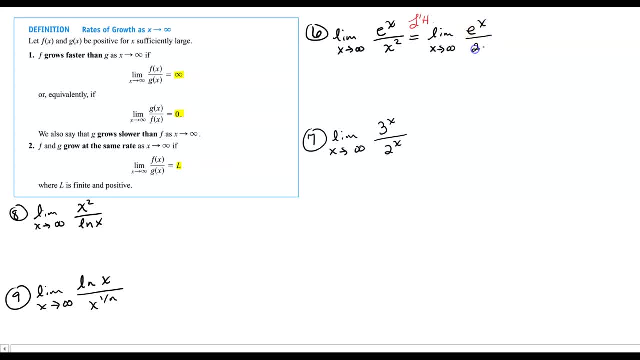 of e to the x is itself e to the x, but the x squared becomes two x. We still can't, you know, plug in infinity. We can't evaluate the limit because it's still indeterminate. We have an infinity over. 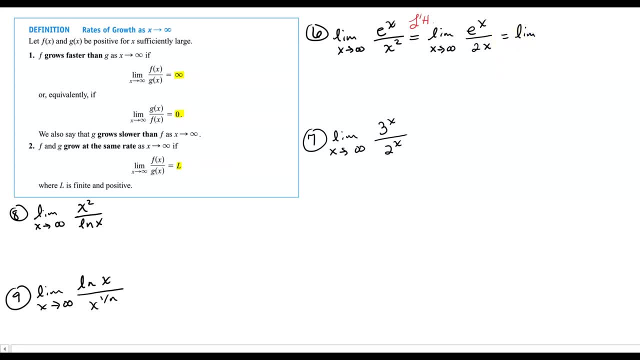 infinity scenario. So we're going to take L'Hopital and apply it one more time, All right, And let's see what we get. We get the limit as x approaches infinity, of what? Well, again it's going to be e to the x, in this case over two. Now we can no longer take. 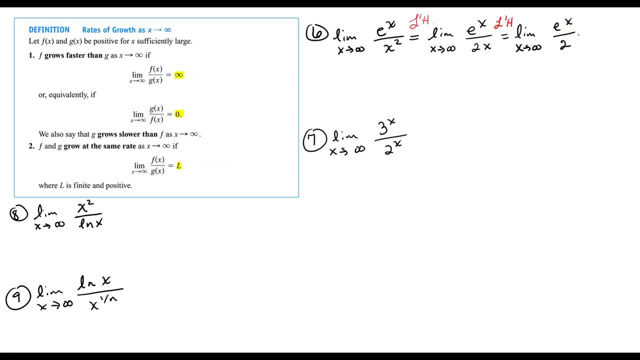 the derivative. Now we can evaluate this, but think about it this way: This right here would be e to the infinity, a huge number divided by two. So what this limit ends up being itself is infinity. Okay, The limit in this case, you know, doesn't exist. All right, So what we can say here? 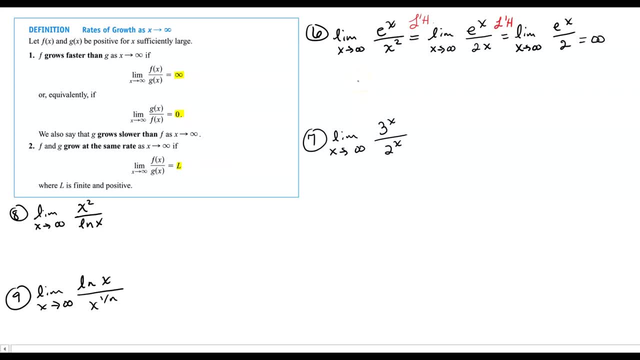 if we're comparing e to the x to x squared, is that, because of this result, f grows faster than g. In this case, e to the x grows faster than x squared. All right, So that's the comparison that we can make. All right, So that's the answer there. All right Now. 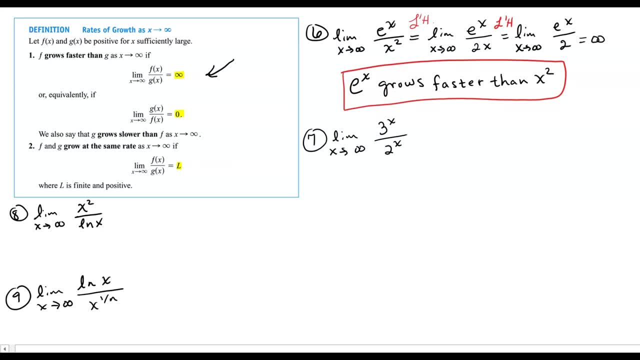 let's take a look at the next one, number seven. We have the limit, as x approaches infinity, of three to the x, over two to the power x. Well, I'm going to not take the derivative. There's no need. This one, I think, can be evaluated. We just have to rethink the way that it looks. So let's take. 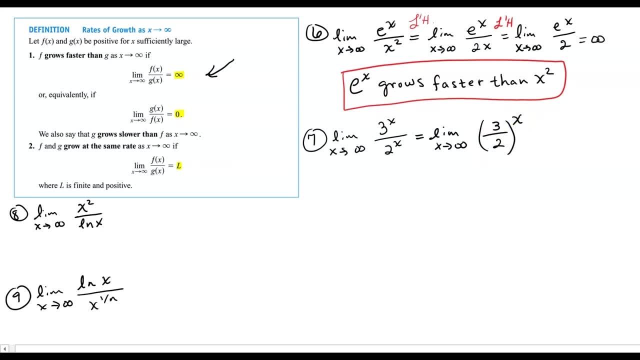 a look at this, We end up with three halves to the power x, because three and two are both being raised to the x power. Well, this is three halves, which is a number greater than one to the infinity power, if you think about it. Okay, So in this case we get infinity again. 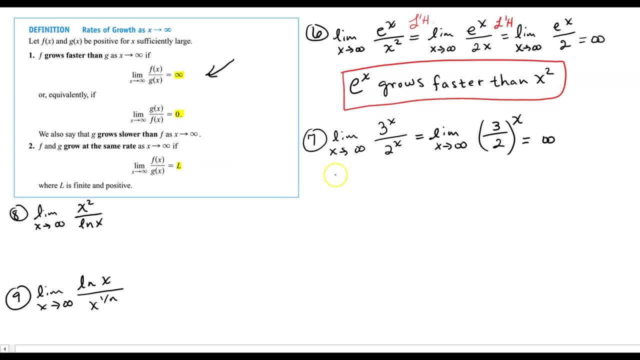 So the answer here- all right, and it should be pretty intuitive- is that three to the x grows faster than two to the x. And think about that for a second. It makes sense: Three to the zero is one, Two to the zero is one, So they're at the same level there. Three to the 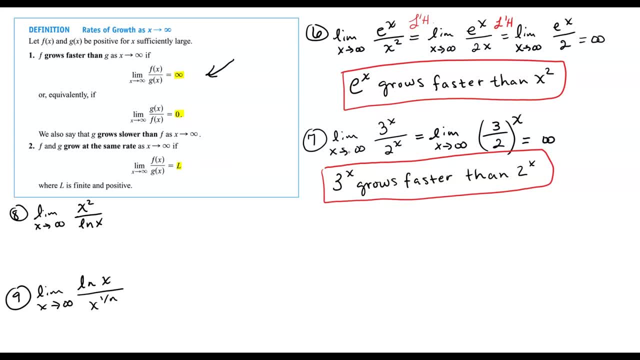 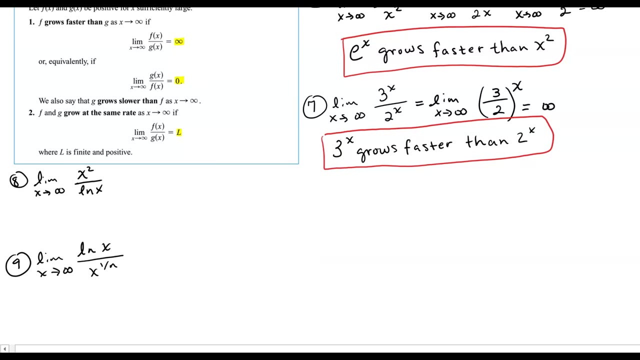 first is three, Two to the first is two. Three is bigger, Three to the second is nine, Two to the second is four. Again the three. the power of three is bigger, So it should make some sense there, intuitively. All right, Let's take a look at number eight here. The limit as x approaches. 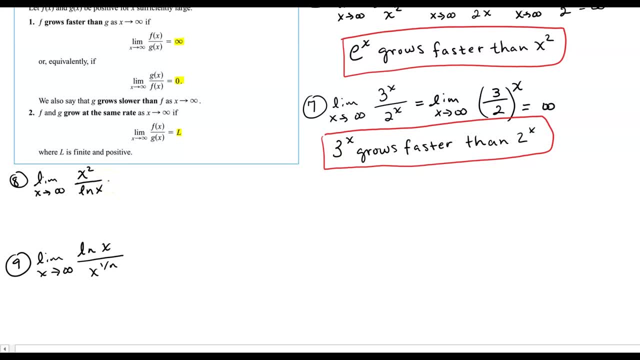 infinity of x squared over the number x. All right, So let's take a look at number eight here: Natural log of x. So this one's an interesting one because we don't know which one grows faster. Now, normally I'd say it's probably going to be the x squared, But let's prove it Only because 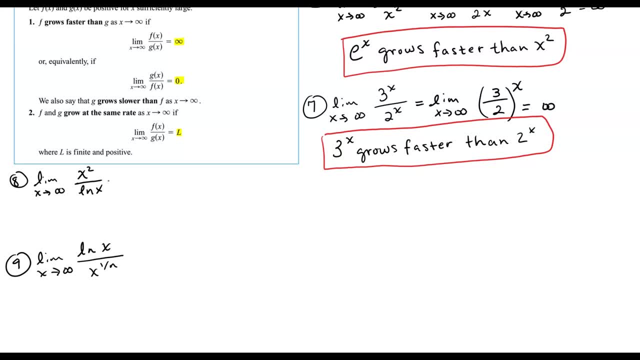 of the statement I made at the very beginning: An exponential function. This one's not exponential. All right, x squared, But exponentials grow faster than logarithms, And I'd imagine that a polynomial would grow faster than a logarithmic. So let's see, Let's apply. 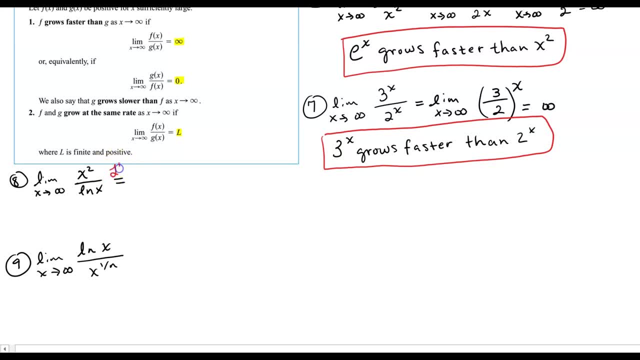 a polynomial L'Hopital's rule in order to get this done. All right, We have the limit as x approaches infinity. Let's take the derivative 2x over derivative of natural log being 1 over x, And we can rewrite this. This becomes the limit as x approaches infinity of 2x squared, Because this: 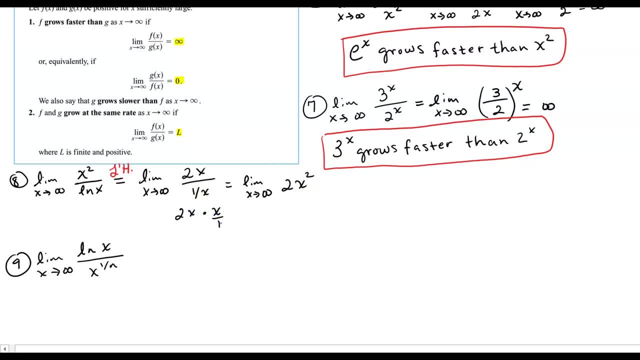 is x multiplied by x over 1.. All right, Keep the first. flip The second. change the sign from division to multiplication. Well, when you evaluate this limit, you end up getting yet again infinity. All right. So it's pretty clear then that x squared grows faster than 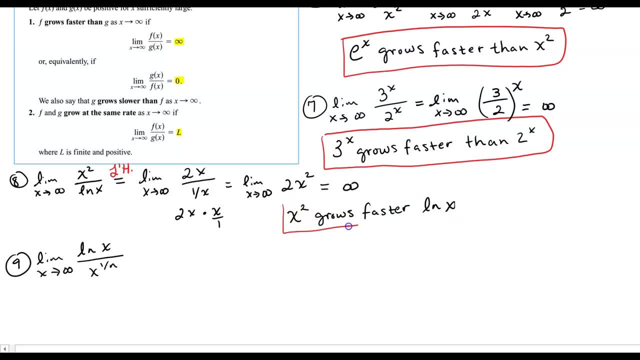 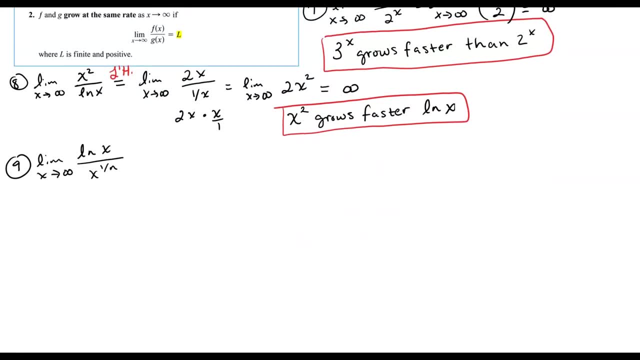 the natural log function, All right. So just keep that in mind. That's how we would do it, All right. One more example: here We're comparing in this case the natural log of x to x to the 1 over n power. All right. 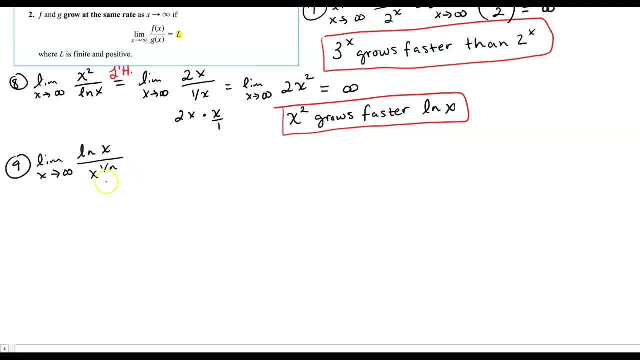 So this is kind of like a general, like a root power, if you will like a root. We're going to compare, We're going to use again L'Hopital's rule, because we need to do that in order to evaluate this limit. We're using n all right as some degree And we're looking 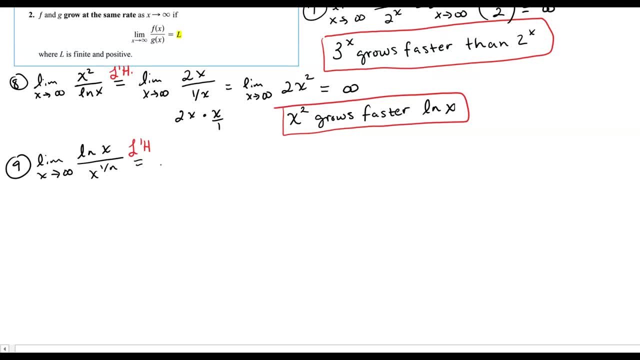 at a power, or x squared x to a certain power and the natural log of x. Let's see The limit as x approaches infinity. I know I have 1 over x. And then the bottom, the denominator is just a power. 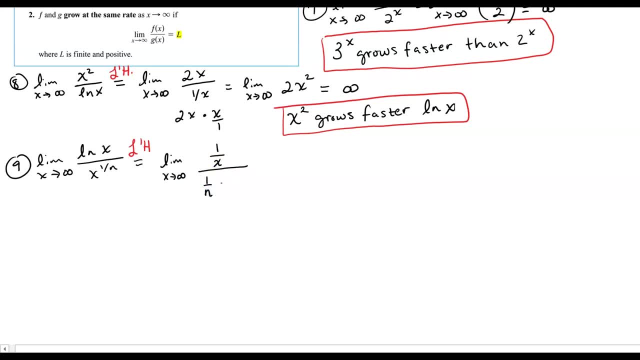 rule problem: Bring down the power x to the 1 over n. 1 over n comes down. x to the power 1 over n minus 1.. All right, x to the power 1 over n minus 1.. All right, What does that? 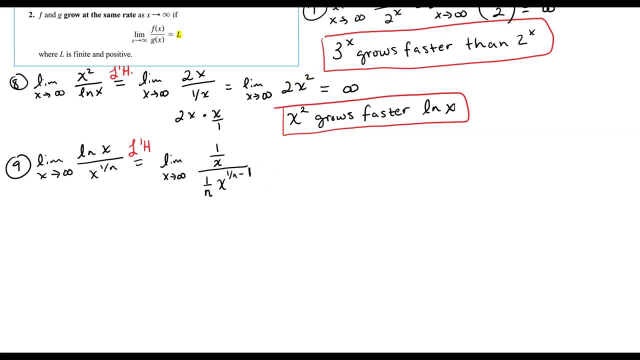 look like: Well, we can simplify this with a little bit of algebra. And what does that look like again, Let's see. All right, We end up with 1 over 1 over n. All right, The 1 over x is really an x to the first power or x to the minus 1, but it's in the denominator. 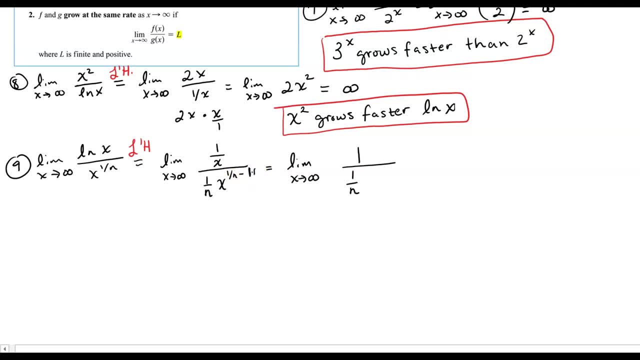 So we end up with a plus 1 scenario here down here, Leaving us with x to the 1 over n power. Okay, Well, think about it. Okay, Think about it: 1 over n. x to the 1 over n is in the denominator. It's a power. Okay, It's a variable.